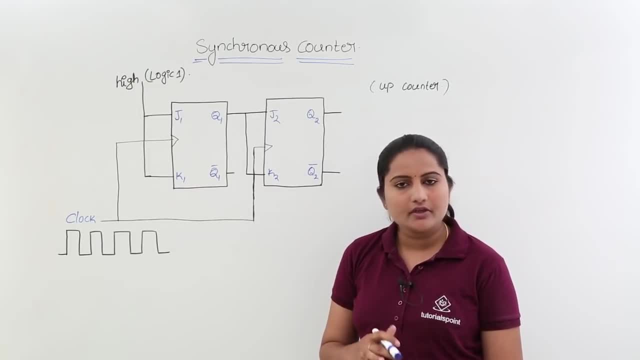 clock is not predefined. inputs are predefined for each and every flip flop. You can observe that class There. we taken this high voltage line to each and every flip flop. We connected that high voltage line to each and every flip flop. that shows you. 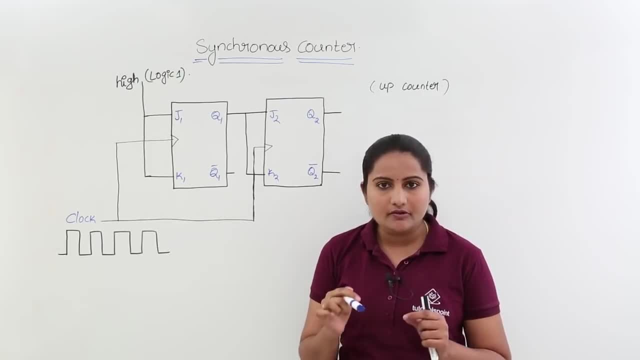 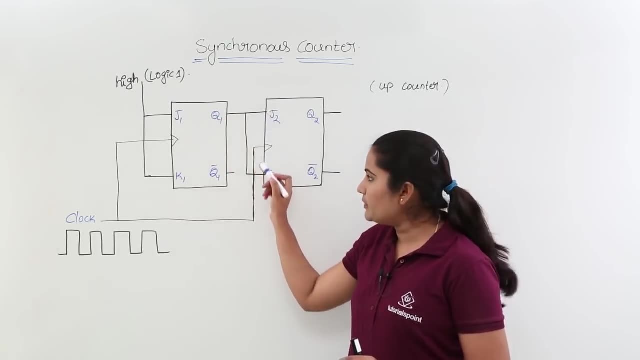 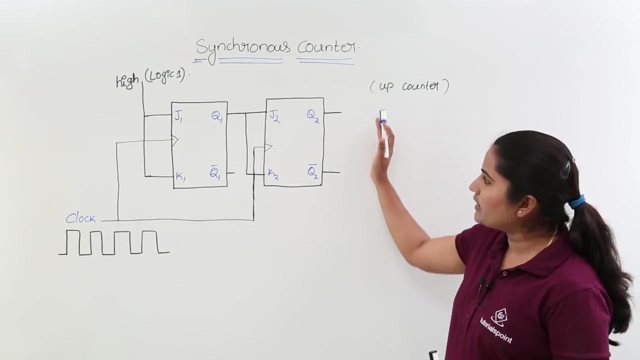 That inputs of each and every flip flop is predefined but clock we are taking from previous flip flop in asynchronous But in synchronous. so here the inputs, the inputs are dependent upon the previous flip flop. For example, 3 bit synchronous counter is there you will. 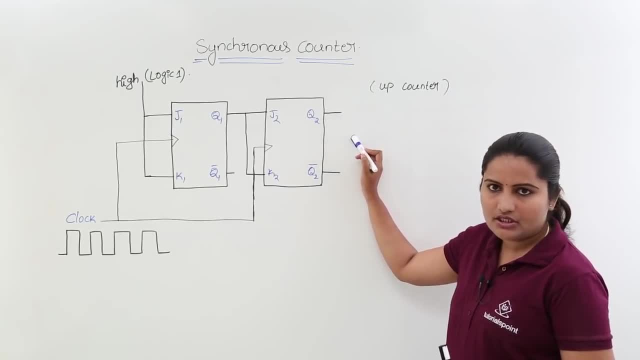 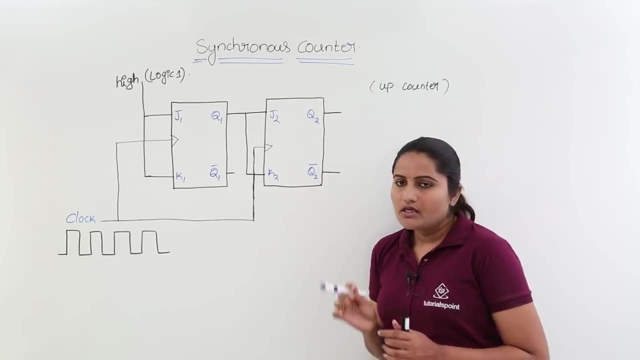 get another flip flop here And whatever this connection is there, we are giving this as input to third flip flop and same clock we are maintaining to that flip flop. So this is about synchronous counter. So this is generally a up counter, synchronous up counter. How it will work like a up counter. 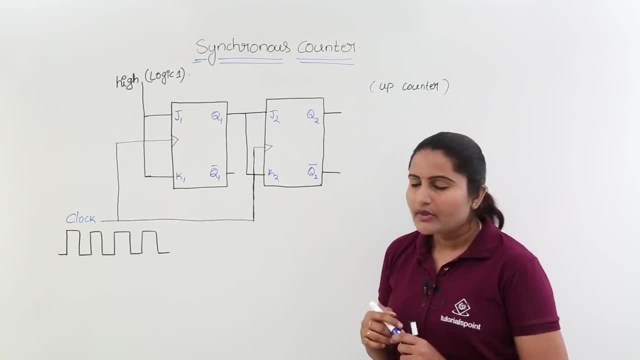 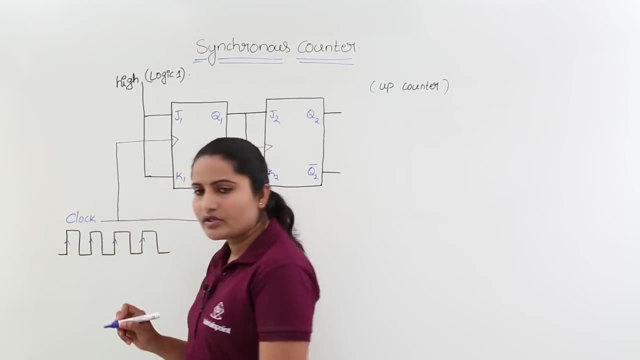 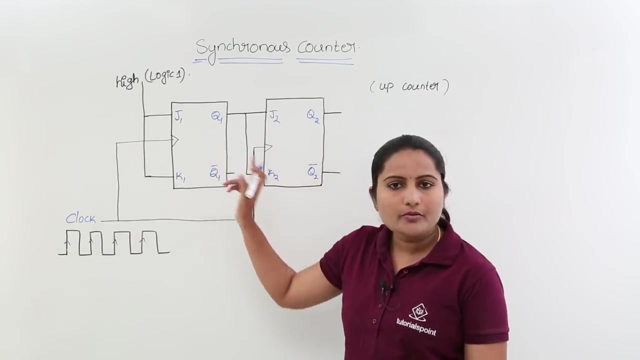 how it will count up counting we will see now. So I am taking positive edge triggered clock now. I am just considering positive edge triggered clock. That means whenever you got positive edge of clock, then these flip flops are going to trigger at a time. Please keep in mind when processing asynchronous circuit, no need to get or no need to worried about inputs and all these One by one you can flow. But when you are dealing with synchronous clock, same clock, then always you need to get ready with the inputs at flip flop side Whenever clock occurred. 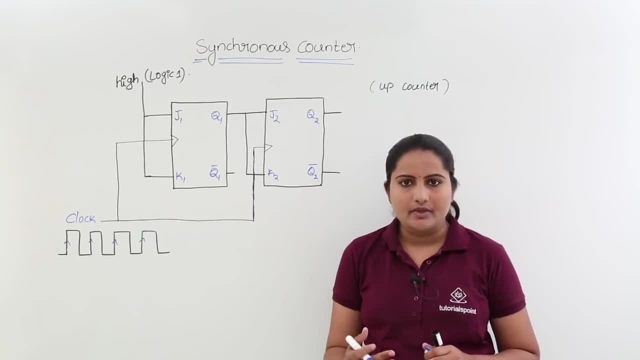 each flip flop will provide output at same time. But in case of asynchronous, you are not doing like that. So first flip flop you are processing, and according to that you are processing second flip flop, and according to that you are processing third and up to n. But in case of synchronous, as clock is similar to each and every flip, 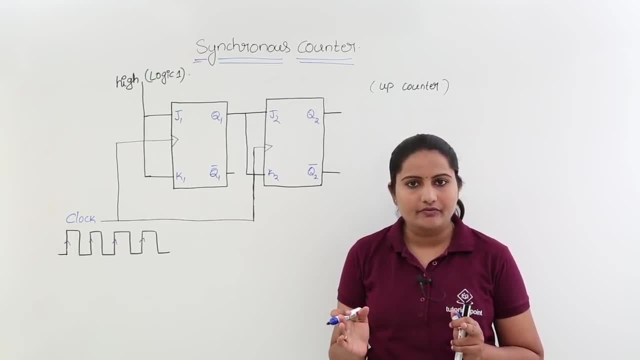 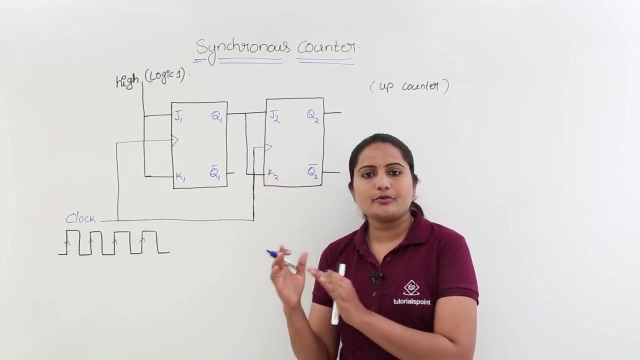 flop, so clock edge is also similar to each and every flip flop. For similar clock edge that means for first clock edge automatically. all flip flops are going to handle their process. That means you need to get ready with the inputs Whenever clock occurred. you need to. 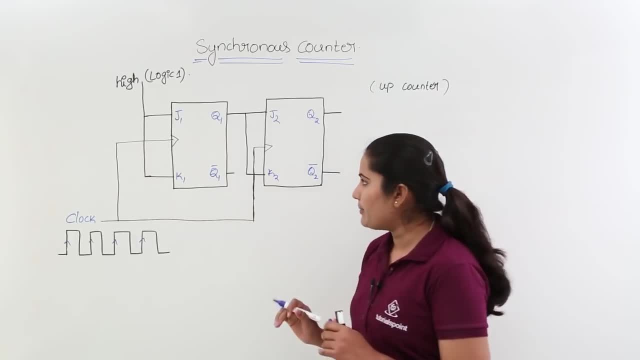 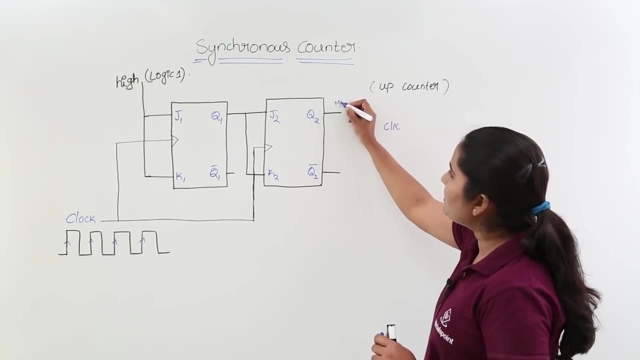 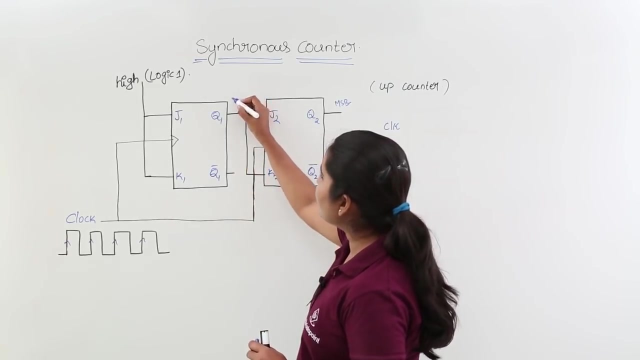 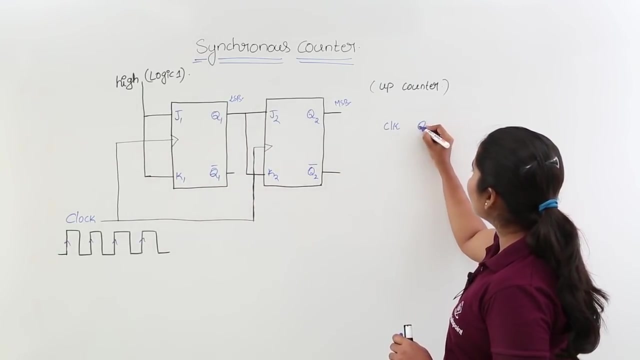 provide the output according to the inputs. Now I am processing that. So here I am considering my clock and, as I told you, MSB will be rightmost side for any counter, either that is asynchronous or synchronous, and LSB will be like this, So that means leftmost. So here clock and Q2,. 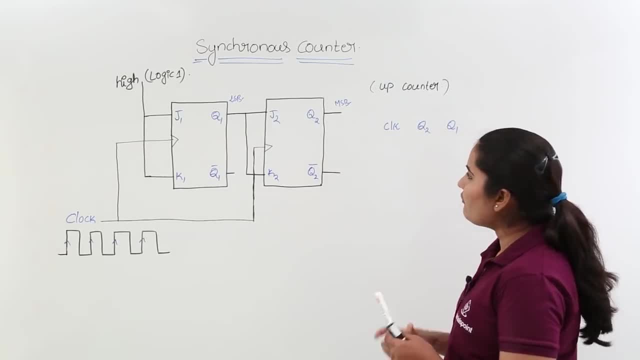 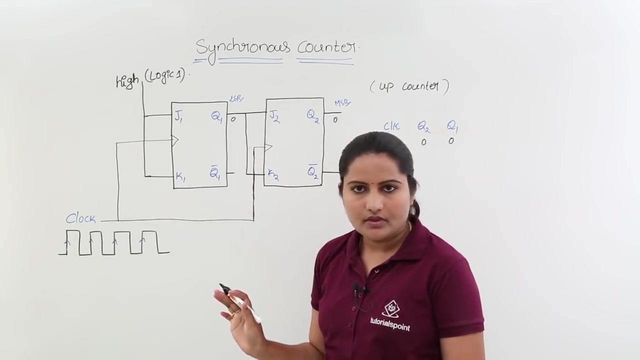 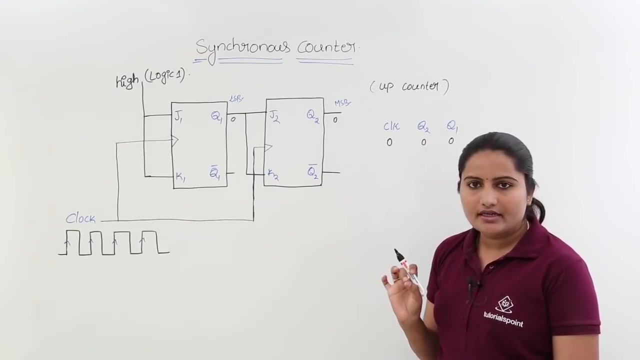 Q1. I consider like this: when clock is equivalent to 0- see here- when clock is equivalent to 0 initially, there is no value in counter. say so, initially we are not having any value in the counter. so while the time of giving first clock pulse, we need to get ready with the possible inputs for this two flip-flops. 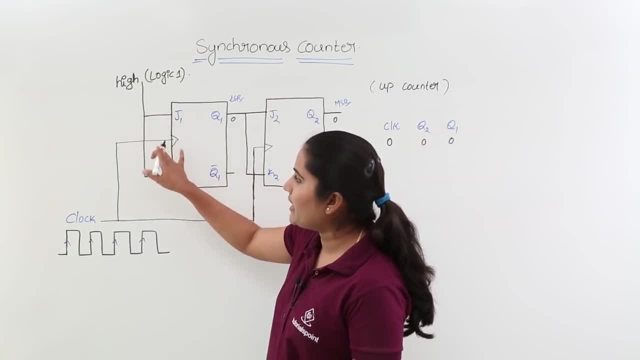 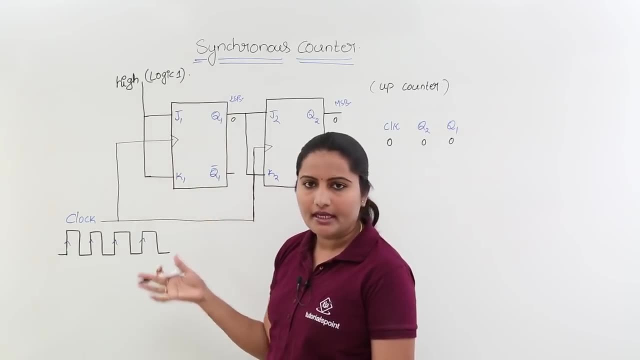 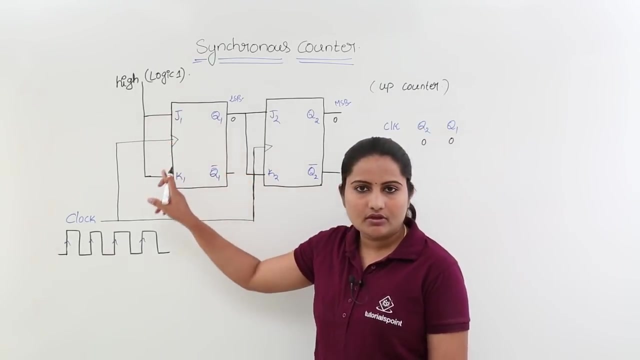 for this flip-flops. what are the input every time? no need to keep in mind about input for first flip-flop because we make it as logic one every time, but for this we need to get ready for inputs. so for this, every time this is equivalent to 1: 1 but for this now. so before. 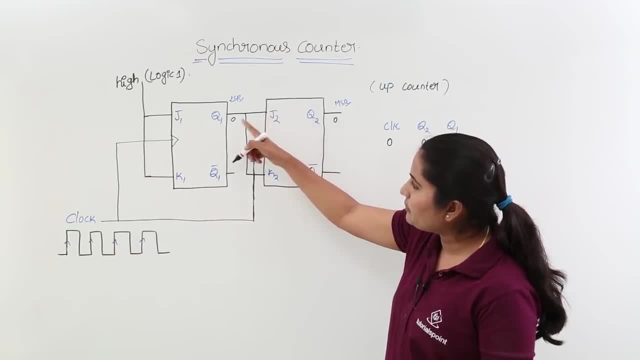 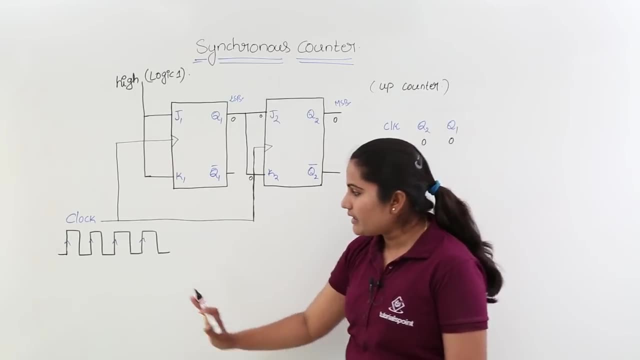 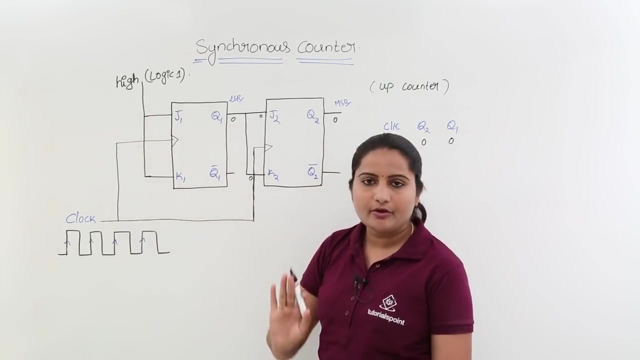 giving first clock pulse, we need to get ready with input means. here initial condition is 0, that 0 will resembles here. So whenever clock pulse is there, whenever we given clock pulse, as the inputs are 1, 1 for JK flip-flop, this is going to toggle. but even though the clock pulse occurred here also. but 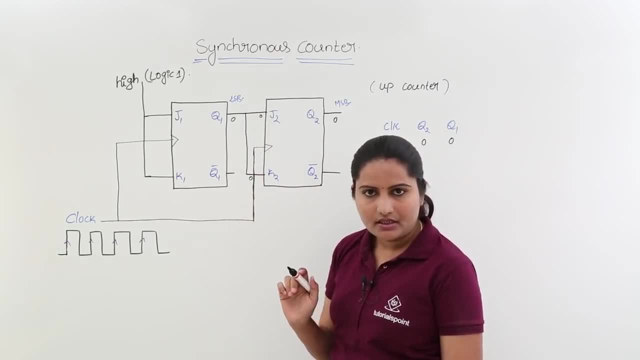 the inputs are 0: 0 for first clock period. this is remains in the same state because you know the JK flip-flop operation if clock is activated for JK flip-flop, if JK is still into the initial state principles. So basically for JK value this 0: 0, it will. it will gives you no change state when JK equal. 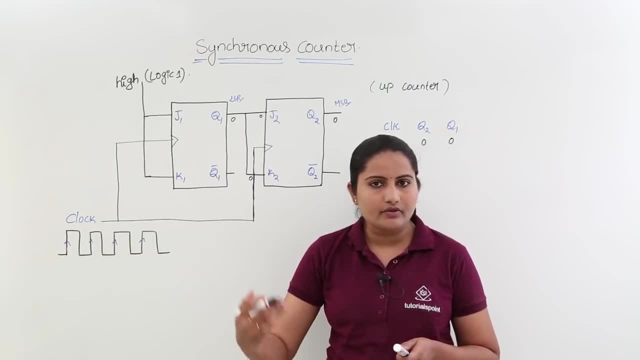 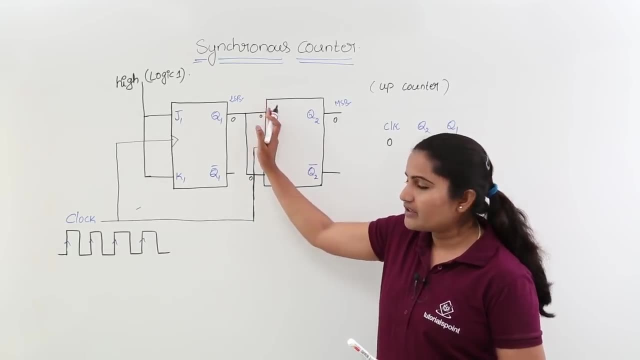 to 0: one, it will gives you reset state. then JK equal to 1: 0, it will gives you set state. when JK equal to 1: 1, it will gives you toggle state. so like that, if you are ready with 0: 0 for first clock pulse, it will gives you no change state. that means 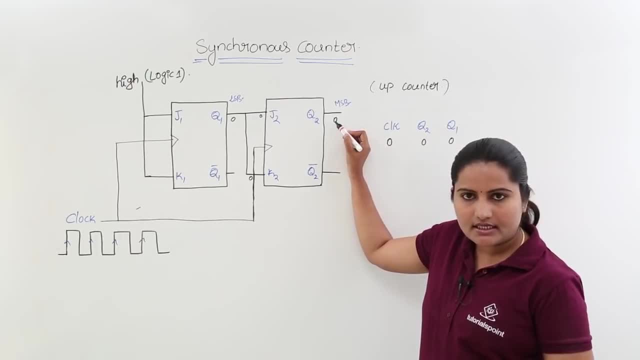 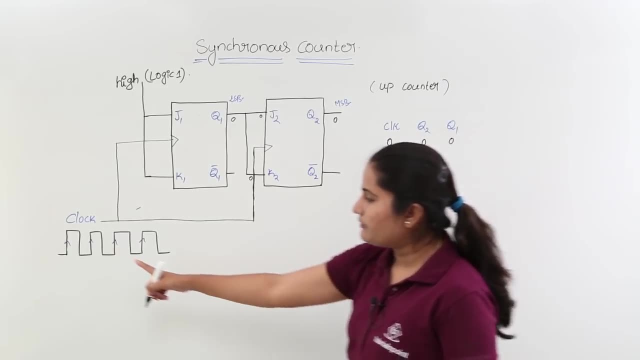 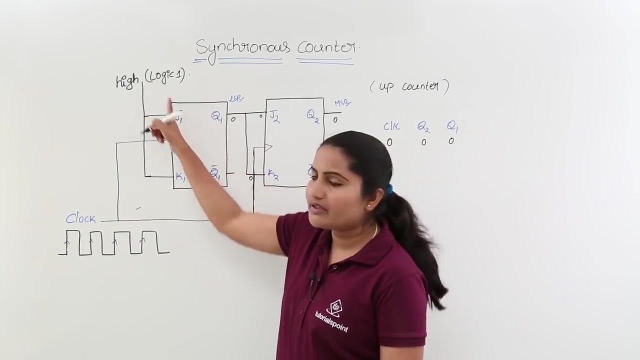 So whatever output state is there- present state is there, that will continue, and previous next state: first clock pulse first. first rising edge. this rising edge will activate both flip-flops, but this flip-flop is ready with 1: 1. so this is going to toggle from 0 to 1, but this is ready. 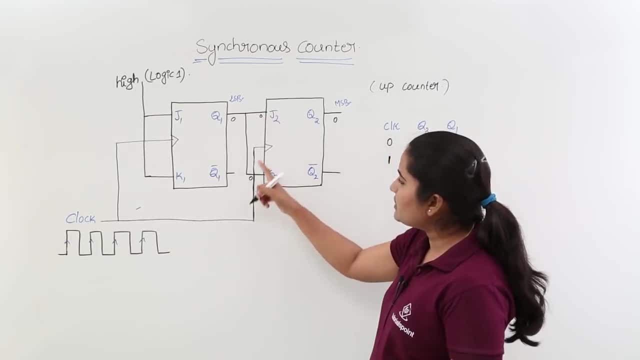 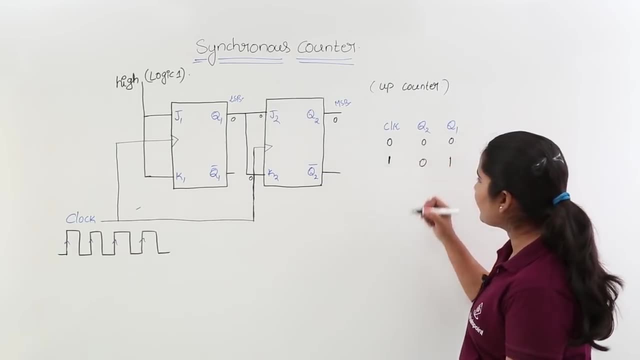 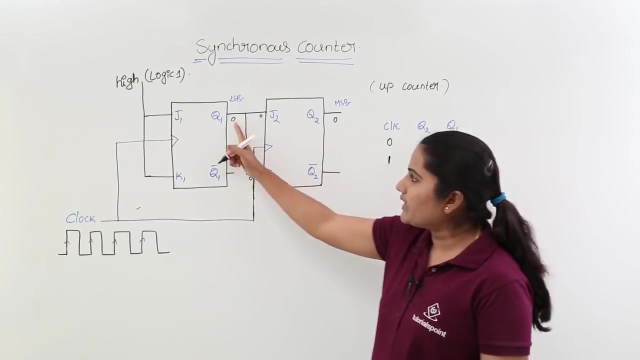 with 0. 0, so this is ready with 0. 0 means so you are getting unchanged output. that means whatever 0 is there, you are getting that 0. so now you got. you may get doubt like this: you got q1 as 1. 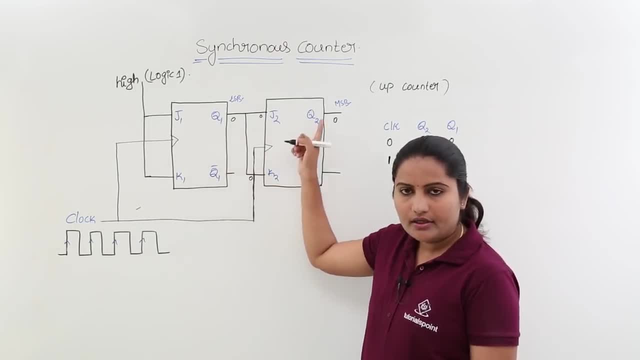 you got q1 as 1, why you can't toggle this flip-flop. this 1 came after application of first clock pulse, so that 1 is available for next clock pulse here. so already same same triggering is applied to this. so this is why you can't toggle this flip-flop, so that 1 is available for next. 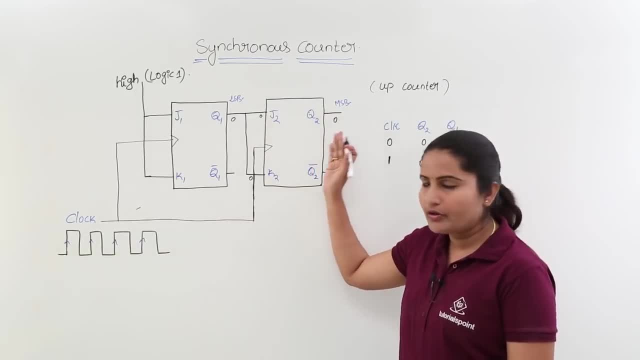 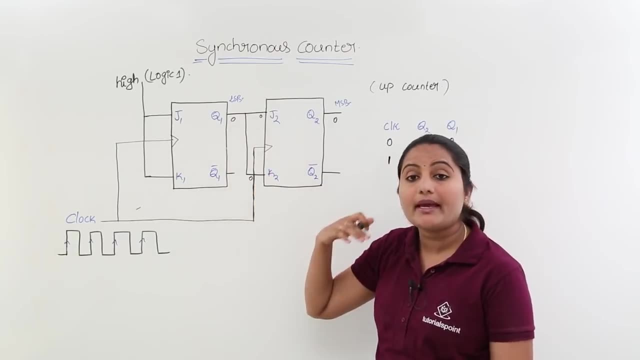 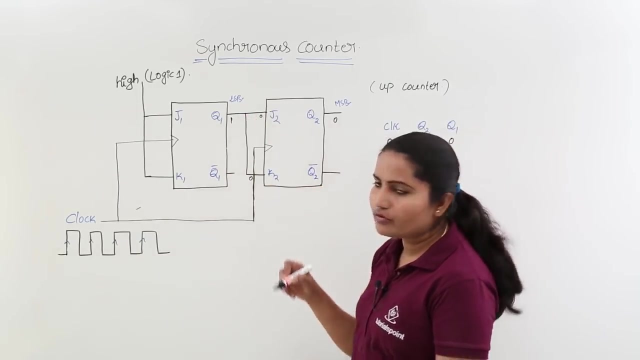 to this flip-flop also. So this already given output when here you got the input. So that means whatever 1 came here, that may be available for the next clock pulse Now. so for first clock pulse this became 0 to 1.. Now here for the next clock pulse application we need. 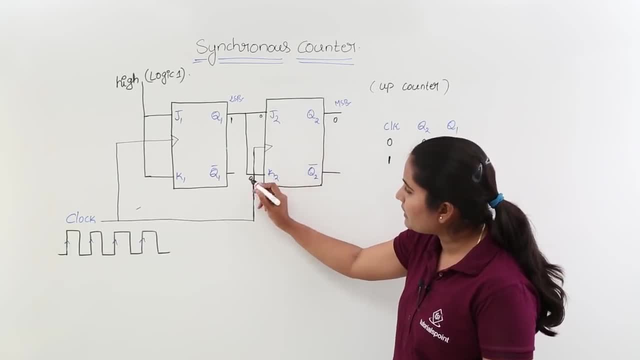 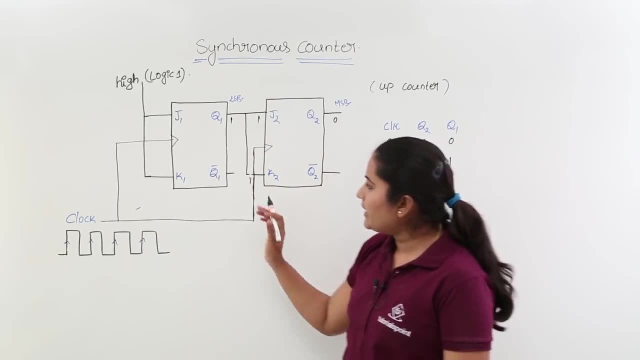 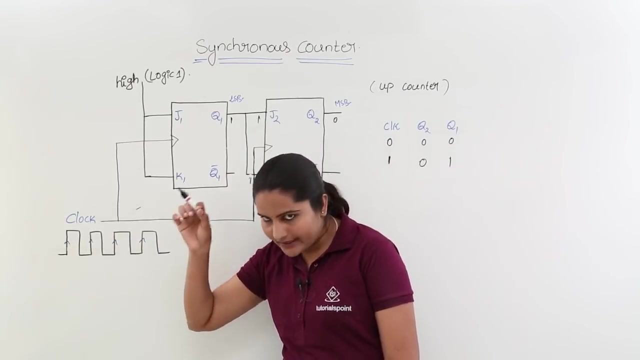 to get ready for the inputs. That means for the second clock pulse application. now it will take 1: 1.. So why it is not taking 1 1 in previous case means so when this edge is there, then only in that edge time these flip-flops are going to work. When this edge 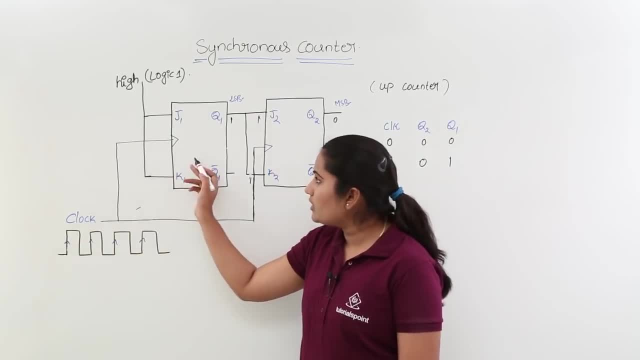 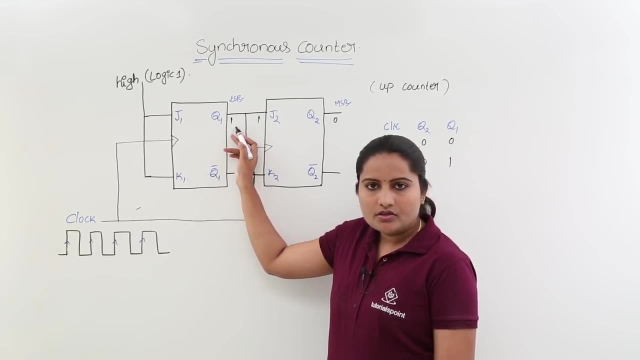 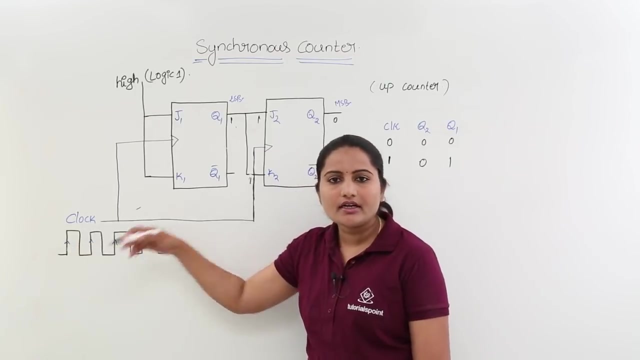 is over. when this edge came, the process time will be there for this flip-flop and it is giving 1.. So to take this: 1.. So this flip-flop is not having this edge. This edge is already completed for this flip-flop. 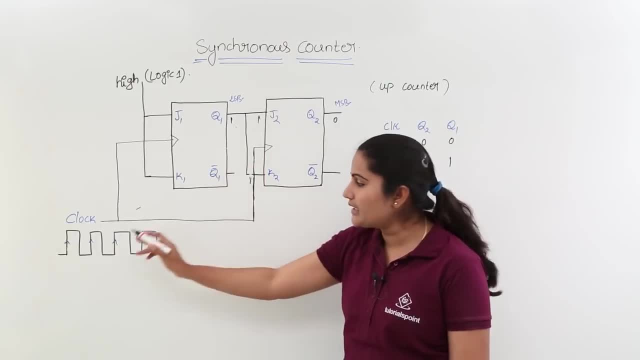 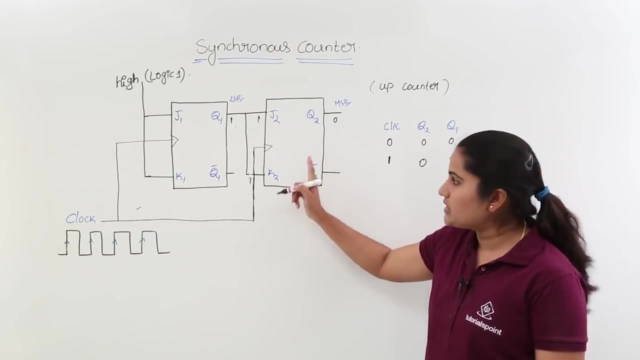 So that is why it will take that value in the next edge. that is the process. So now we will see so for next clock pulse application, our available input is 1, 1, here and here, always 1, 1.. So now I applied second rising edge of clock. I applied second rising edge of. 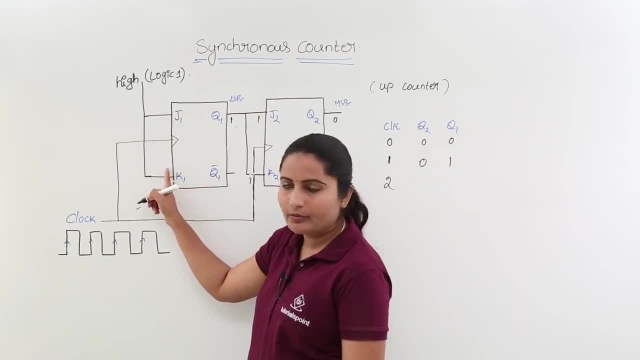 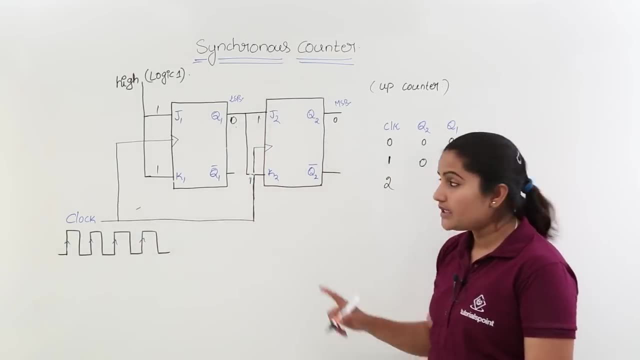 clock 1, 1, having 1, 1 at input. always this is given with 1, 1.. So it is going to toggle from 1 to 0. that 0 will not come here directly because whatever ready inputs are there, that will take. this 0 will come in next clock pulse. So for this clock pulse in second same second clock pulse. for this, for this flip flop, for the second clock pulse: as 1, 1 is there, this is also going to toggle. that means this will become 0 to 1. that means you will get 0, 1.. 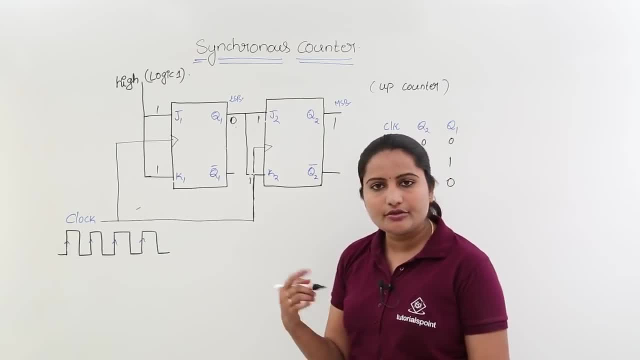 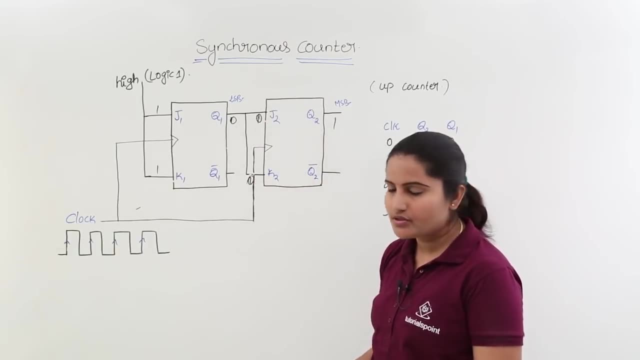 So for application of third clock pulse you need to again ready with inputs. So now it will take 0, 0, now it will take 0, 0, and now you need to give your third clock pulse. So when you given third, 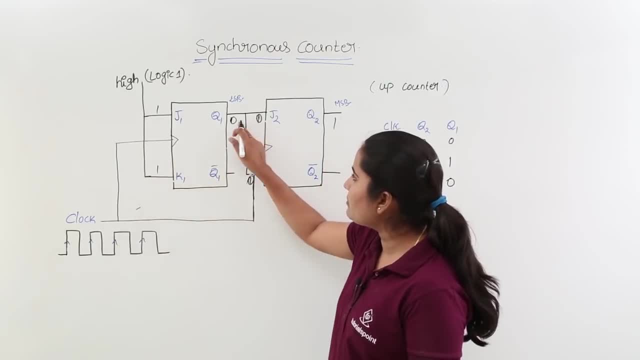 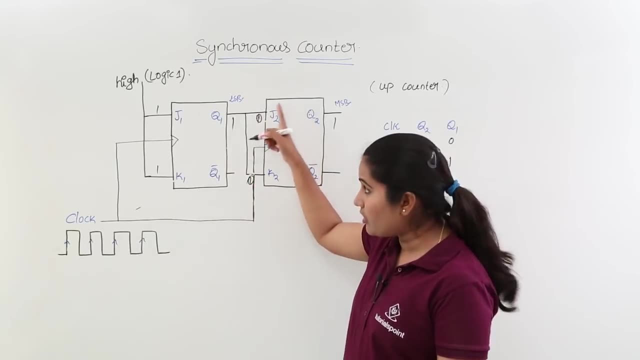 rising edge of clock then it is going to toggle from 0 to 1.. This will become 0 to 1.. So for application of third clock pulse you need to again ready with inputs. So this 1 is not going to here now. this flip flop is not considering 1 now because 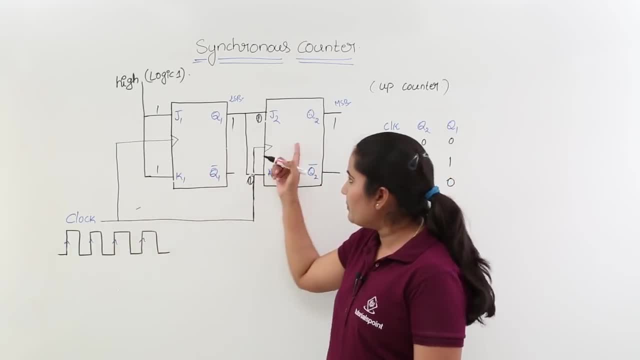 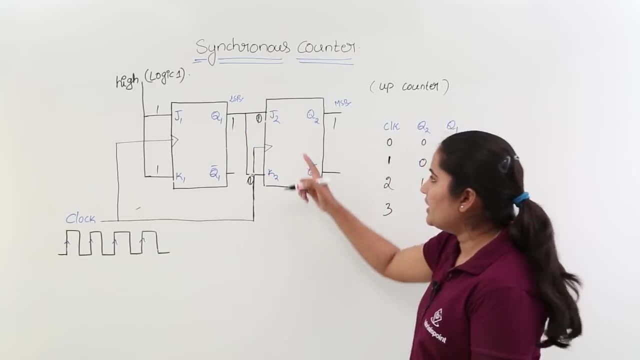 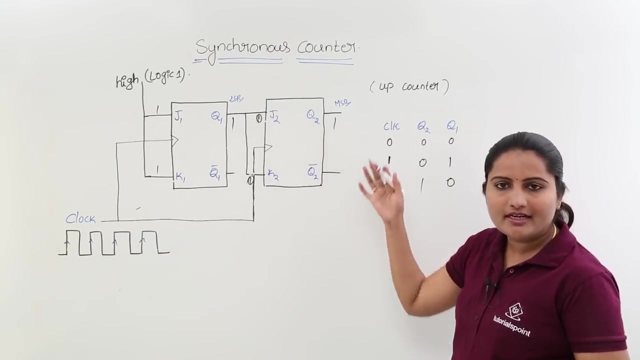 for the third rising edge. the previous inputs are 0: 0. that will come. This 1 will come in fourth clock pulse. So here, whatever 0, 0 is there. for example, if you are giving 0, 0 for JK flip flop, that will provides you no change condition. No change condition means whatever. 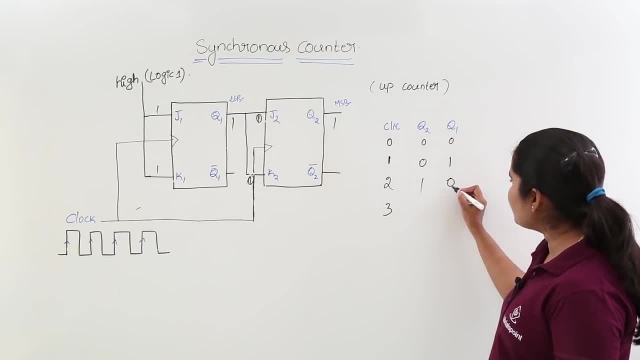 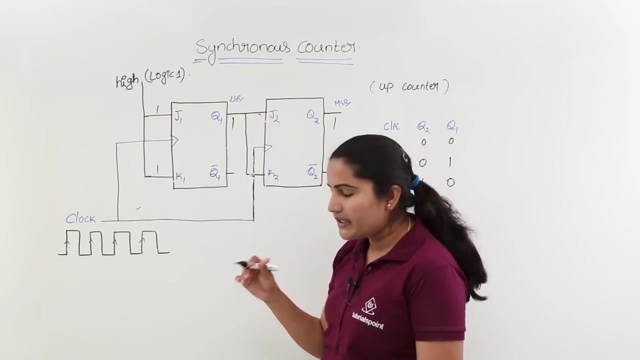 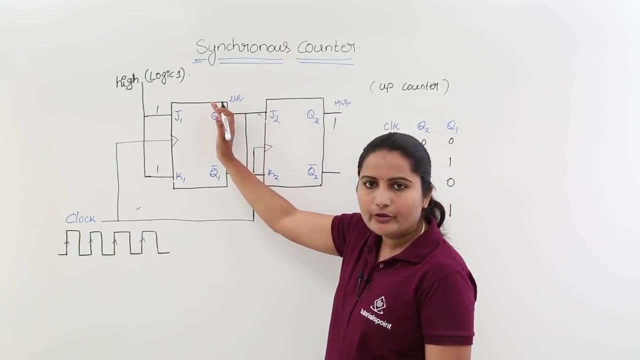 previous is there. that will come as it is. So here this is going to toggle and this will remains as it is. And when you applied fourth clock pulse, then you need to get ready with the input. So for fourth, please keep in mind, for every clock pulse, the input of this flip flop is from output of, output of. 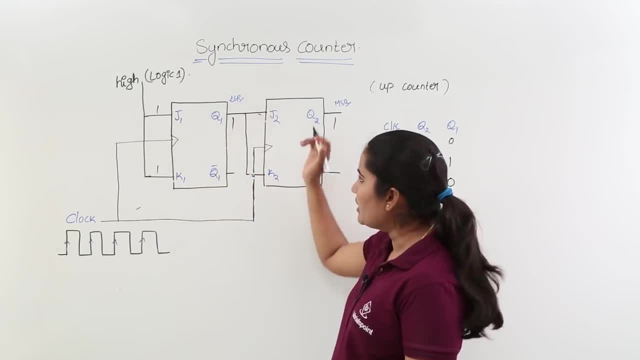 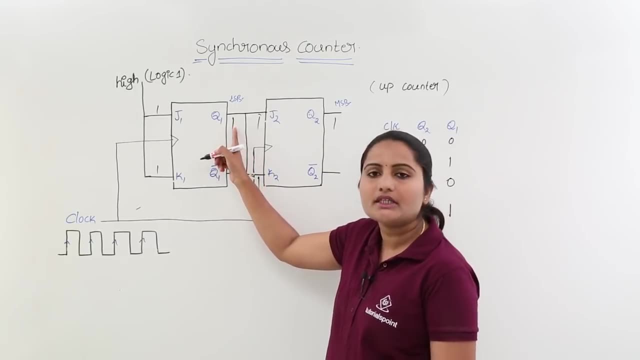 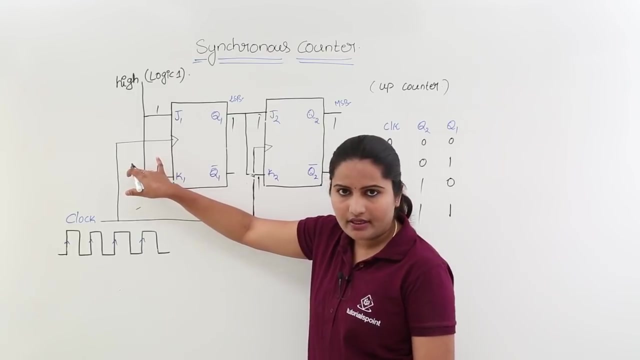 first flip flop generated from previous clock. that is it. So here now for fourth clock pulse. you need to get ready with the input which is generated from third clock. So now we are having 1: 1 here and always here. also we are having 1: 1 here When we applied fourth. 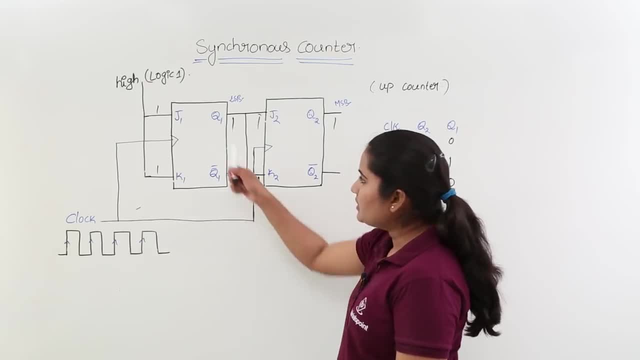 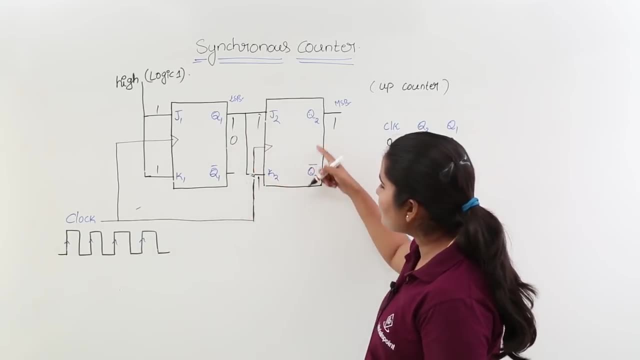 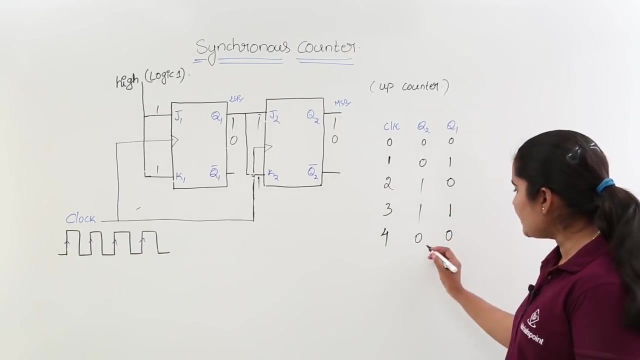 clock pulse. when fourth rising edge came, then this flip flop and this flip flop, both are going to be in toggle condition. It will become 0 and this is also going to toggle means. this will become 0. condition will come. That means if you got 0, 0 means counter will stop counting. 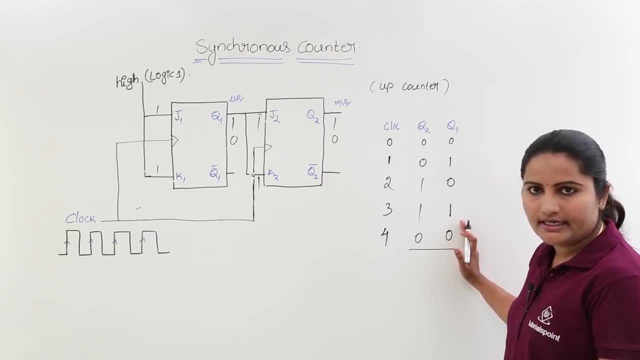 it will shows it is passed through 4 states. That means, as this is a 2 bit counter, we may have 4 states. So you can see 0, 0, 1, 2, 3. this is up counting right, For example, if you 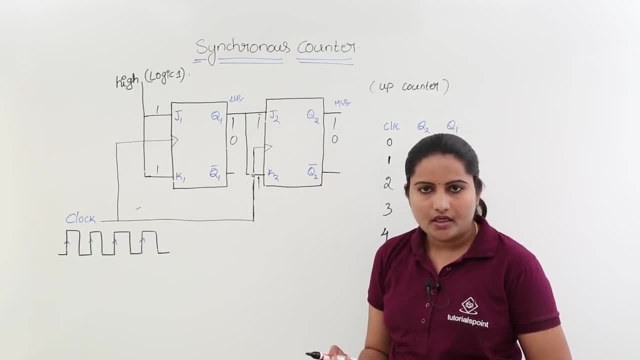 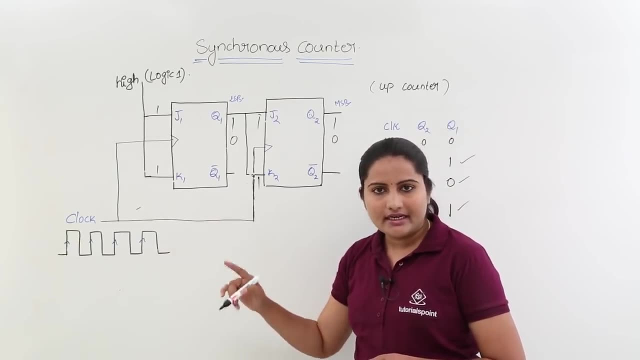 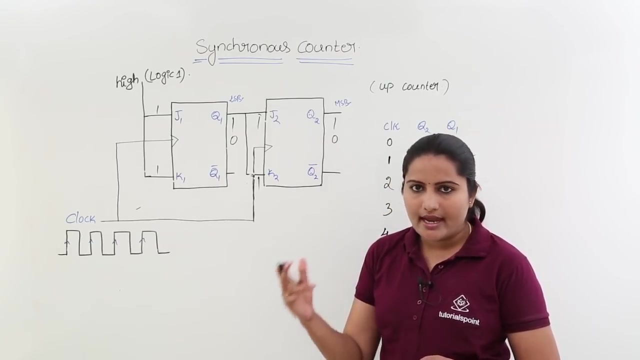 want to use same circuit for a down counting. if you want to use same circuit for a down counting, So you change this clock to negative edge triggered clock. negative edge triggered clock means So 0 is going to activate the flip flop up to now. if 1 is there, then it is going. 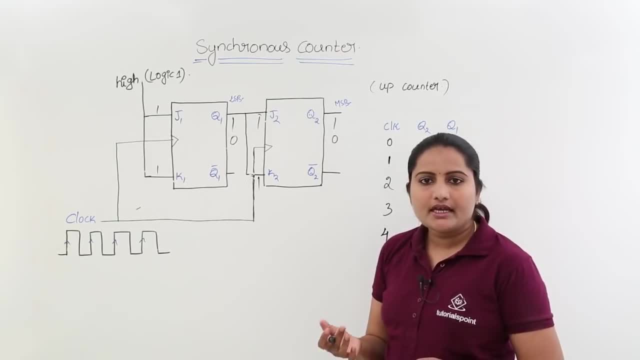 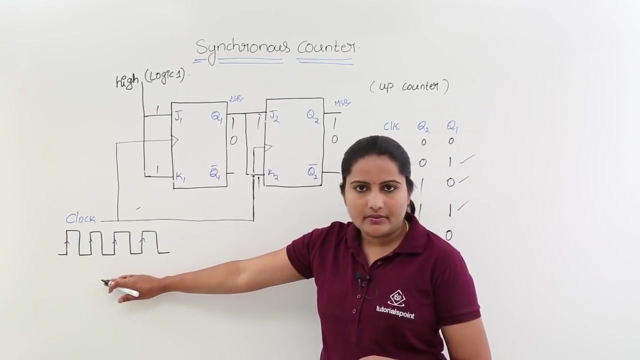 to activate the flip flop. but if we consider negative edge triggered flip flop then sorry, negative edge triggered clock, then it shows you 0 will activate the flip flop. So, or with the same clock, that means with the positive edge triggered clock, if you want to make the circuit as down counter, then you need to change the connection from here to here, That means from q 1 bar to j 2, k, 2. you need to connect like the like that you can generate synchronous down counter. just by changing the connection you can generate synchronous down counter. .